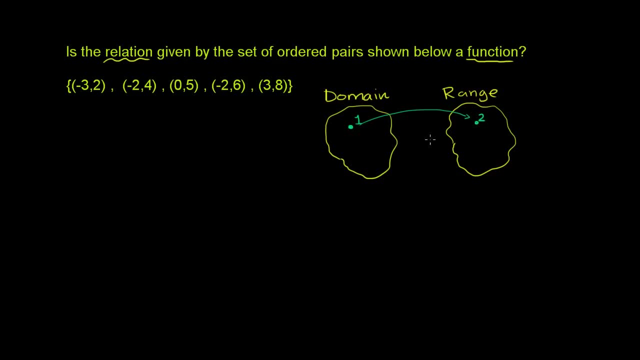 with the number 2 in the range. So in this type of notation you would say that the relation has 1 comma 2 in its set of ordered pairs. These are two ways of saying the same thing. Now the relation can also say, hey, maybe if I have 2,. 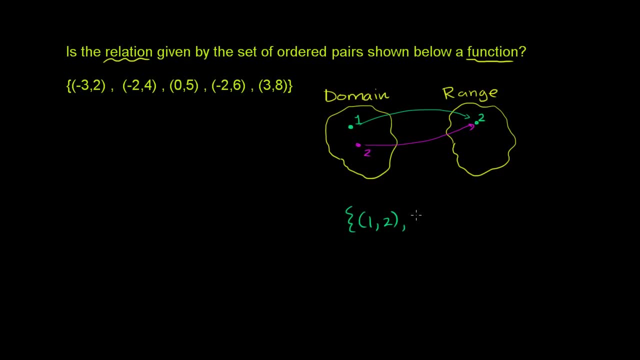 maybe that is associated with 2 as well, So 2 is also associated with the number 2.. And so notice, I'm just building a bunch of associations. I've visually drawn them over here Here. I'm just doing them as ordered pairs. 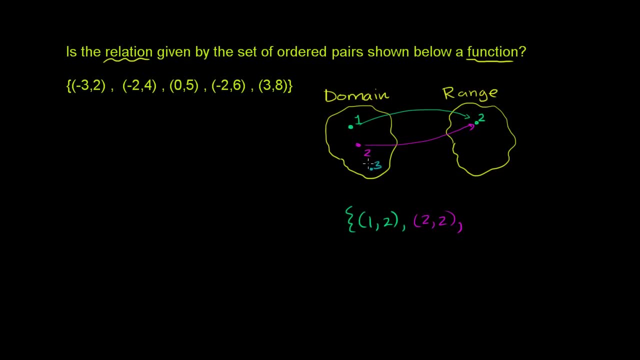 We could say that we have the number 3.. 3 is in our domain. Our relation is defined for number 3. And 3 is associated with 2. And 3 is associated with, let's say, negative 7.. 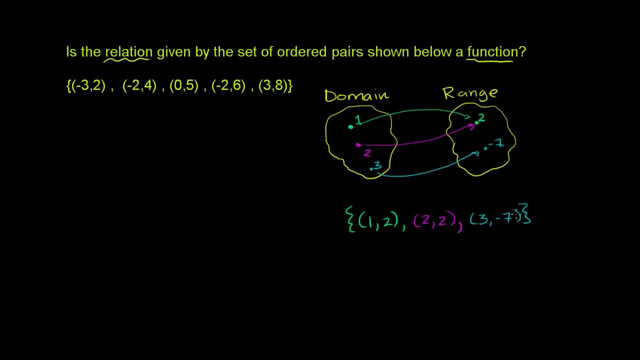 So this is 3 and negative 7.. Now this type of relation right over here, where if you give me any member of the domain and I'm able to tell you exactly which member of the range is associated with it, this is also referred to as a function. 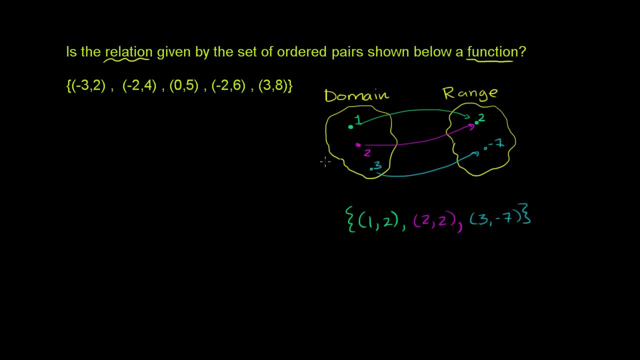 And in a few seconds I'll show you what a relation that is not a function, Because over here you pick any member of the domain And the function really is just a function. It's not just a relation, It's really just an association. sometimes 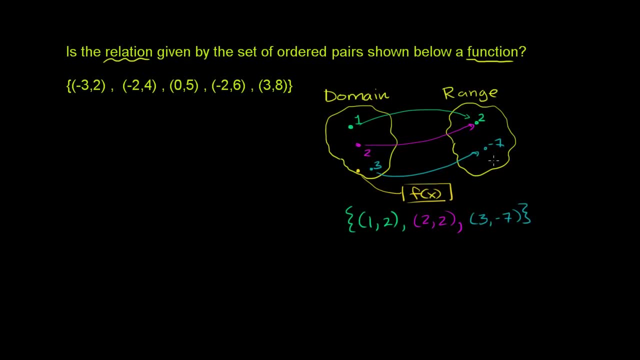 called a mapping between members of the domain and particular members of the range. So you give me any member of the domain, I'll tell you exactly which member of the range it maps to. You give me 1, I say hey, it definitely maps to 2.. 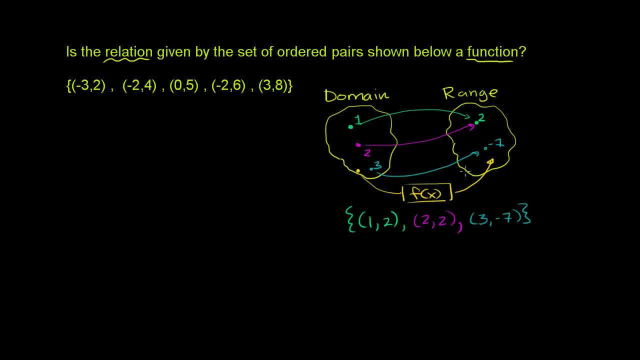 You give me 2, it definitely maps to 2 as well. You give me 3, it's definitely associated with negative 7 as well. So this relation is both a. it's obviously a relation, but it is also a function. 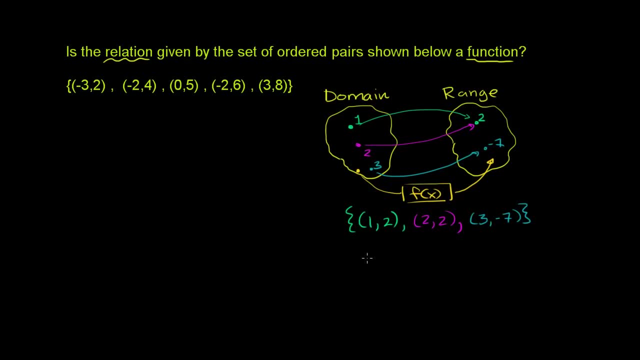 Now to show you a relation that is not a function. imagine something like this. So once again, I'll draw a domain over here And I'd do this big fuzzy, cloud-looking thing to show you that I'm not showing you all of the things in the domain. 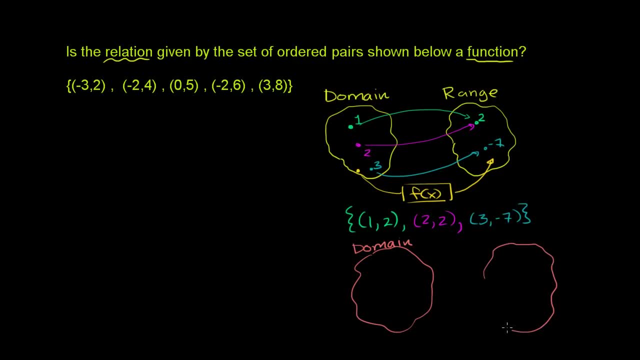 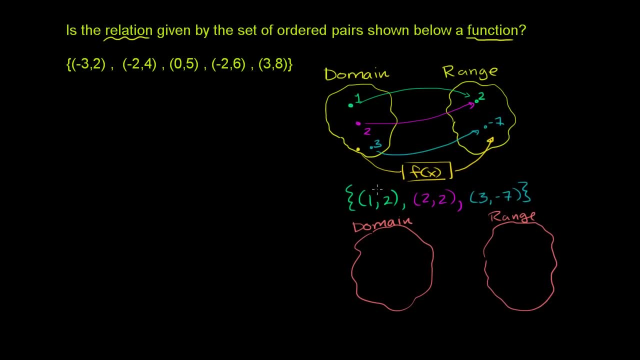 I'm just picking specific examples. And let's say that this big fuzzy, cloud-looking thing is the range. And let's say in this relation- and I'll build it the same way that we built it over here- Let's say, in this relation, 1 is associated with 2.. 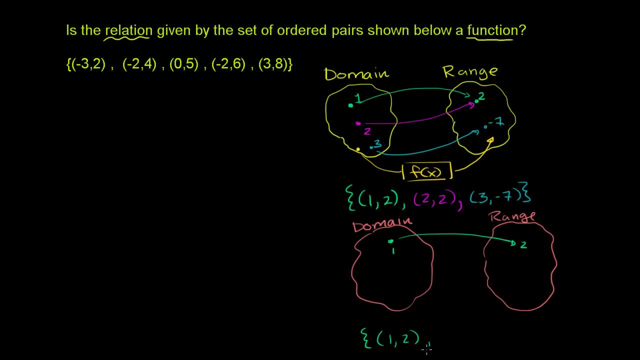 So let's build the set of ordered pairs. So 1 is associated with 2.. Let's say that 2 is associated with negative 7.. Let's say that 2 is associated with negative 3. So you'd have 2, negative 3 over there. 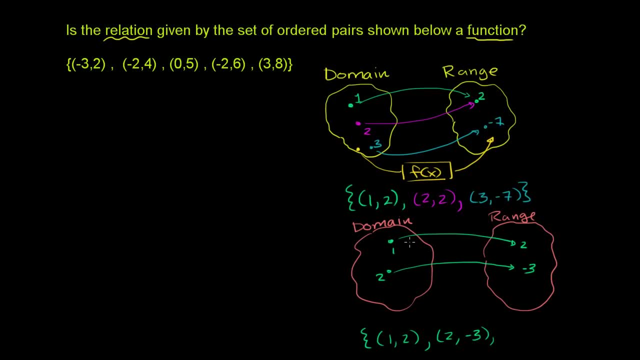 And let's say, on top of that we also associate 1 with the number 4.. So we also create an association with 1 with the number 4.. So we have the ordered pair 1 comma 4.. Now, this is a relationship. 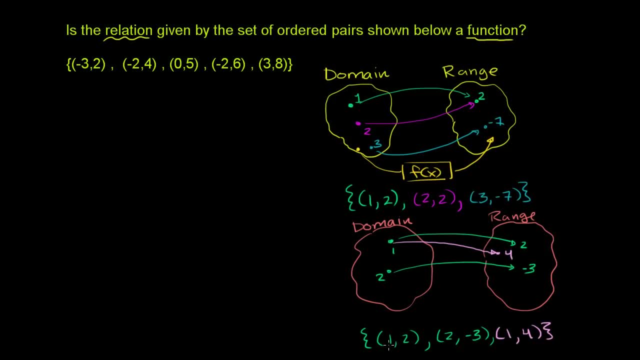 We have it's defined for a certain domain. If this was the whole relationship, then the entire domain is just the numbers 1, 2.. Actually, just the numbers 1 and 2. It's definitely a relation, but this is no longer a function. 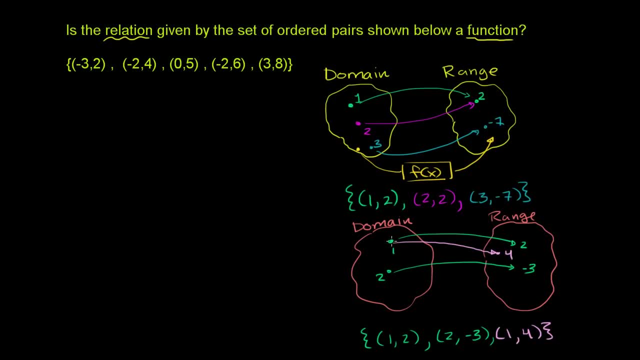 And the reason why it's no longer a function is: if you tell me, OK, I'm giving you 1 in the domain. What member of the range is 1 associated with it? Over here you say, well, I don't know. 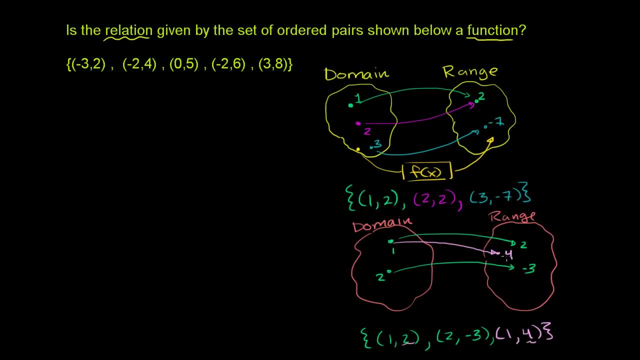 Is 1 associated with 2, or is it associated with 4?? It could be either 1.. So you don't have a clear association. If I give you 1 here, you're like: I don't know, Do I hand you a 2 or 4?? 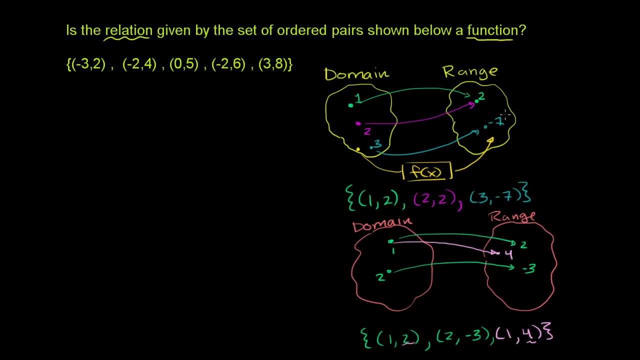 That's not what a function does. A function says: oh, if you give me 1, I know I'm giving you a 2.. You give me a 2, I know I'm giving you a 2.. Now, with that out of the way, let's actually 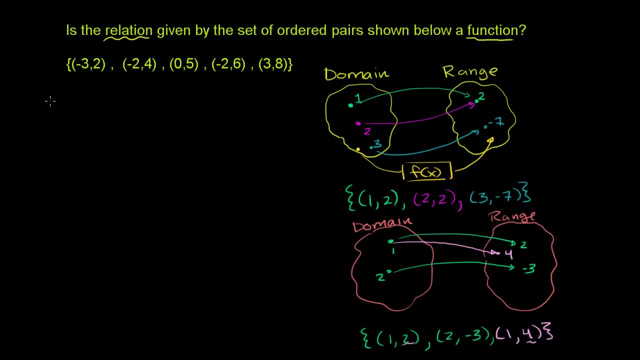 try to tackle the problem right over here. So let's think about its domain and let's think about its range. So the domain here, the possible. you could view them as x values or inputs into this thing. that could be a function, that's. 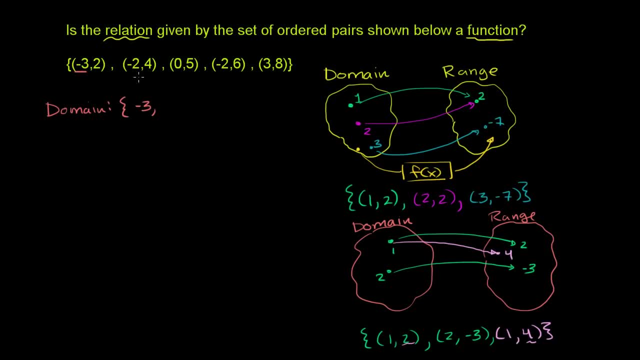 definitely a relation. You could have a negative 3.. You could have a negative 2.. You could have a 0.. You could have a- well, we already listed a negative 2, so that's right over there. Or you could have a positive 3.. 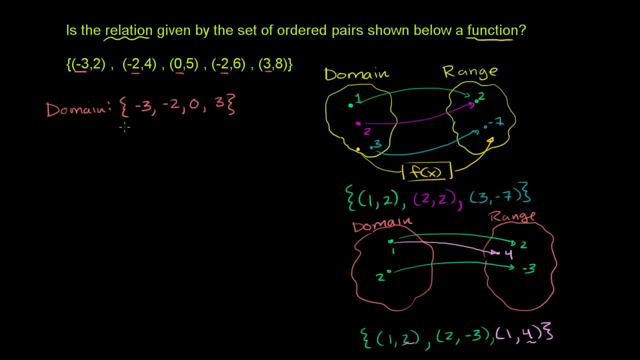 Those are the possible values that this relation is defined for that you could input into this relation and figure out what it outputs. Now the range here. these are the possible outputs or the numbers that are associated with the numbers in the domain. The range includes 2,, 4,, 5,, 6, and 8..